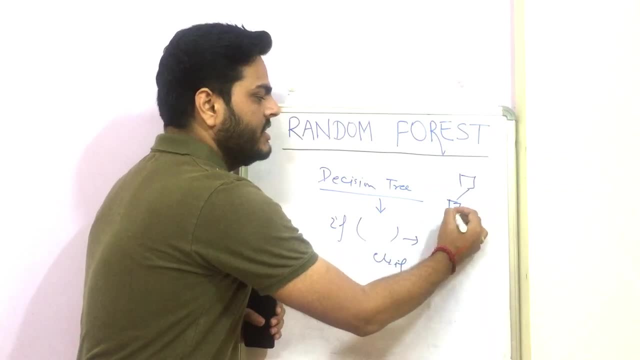 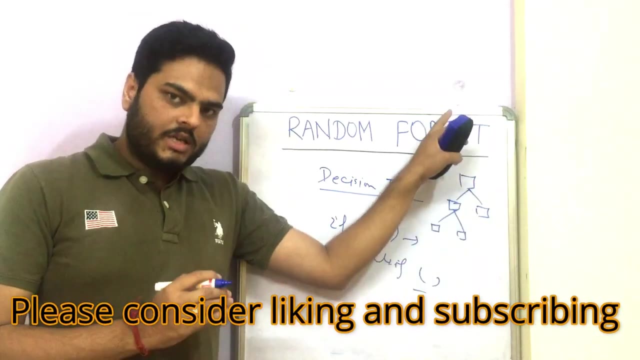 meaning of overfitting is if a decision tree model gets trained like this: So this is the tree and these are the different branches of the tree. So if a tree keeps growing, if a tree keeps growing till the last node or last leaf, then there is a tendency of 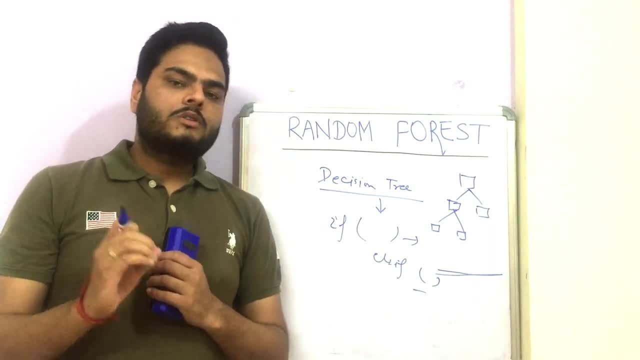 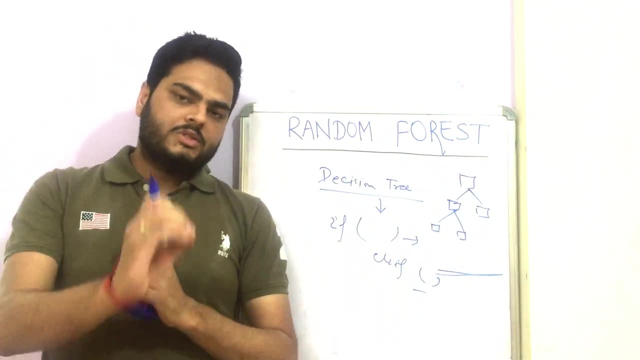 decision tree of overfitting, Or in other words can say high variance. So what is the meaning of high variance is, let's say, this tree gets trained okay, and you want to check the accuracy of the tree on a test data or on an unseen data. So 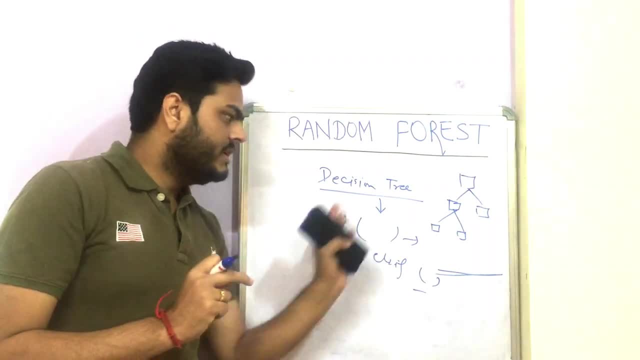 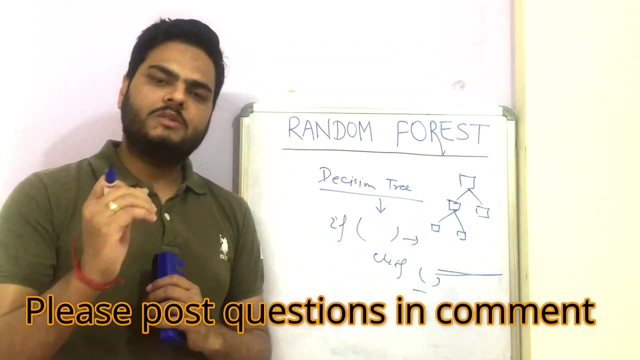 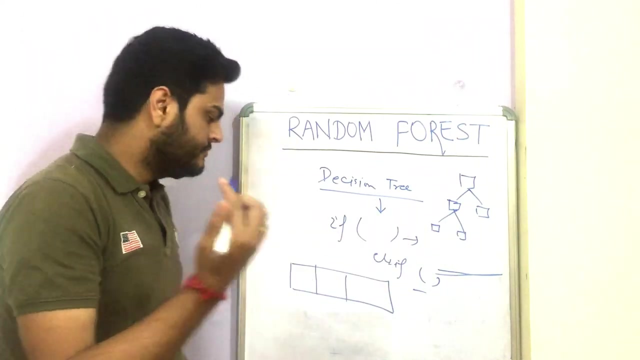 decision tree don't tend to perform very well on test data, which means the training accuracy might be high, but test accuracy will not be high. Let's try understanding with a simple example. So let's say: this is the test data that you want to expose to decision tree, for you know prediction, So let's 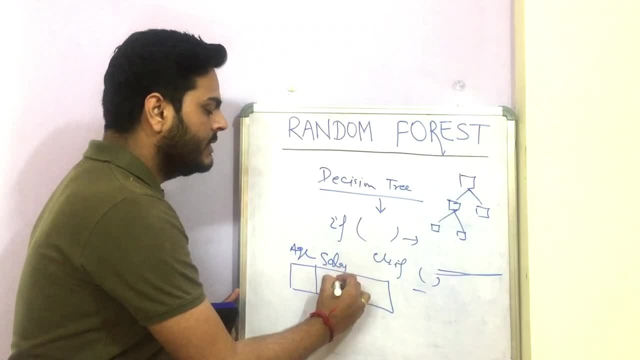 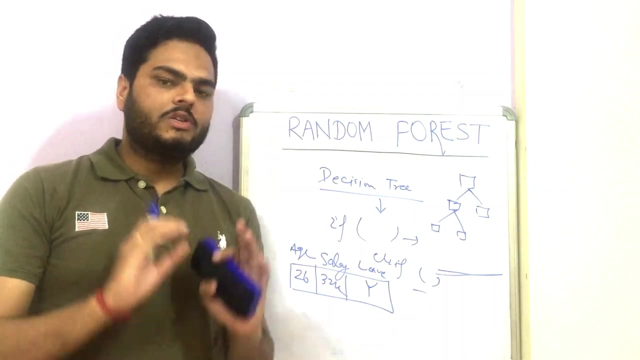 say: this is the age column and this is the salary column, and you want to understand whether the employee will leave or no, okay, So if your age is, let's say, 26 and salary is, let's say, 32k, and then the decision tree may say: leave, yes, okay. but it is quite possible that if you make this 26, 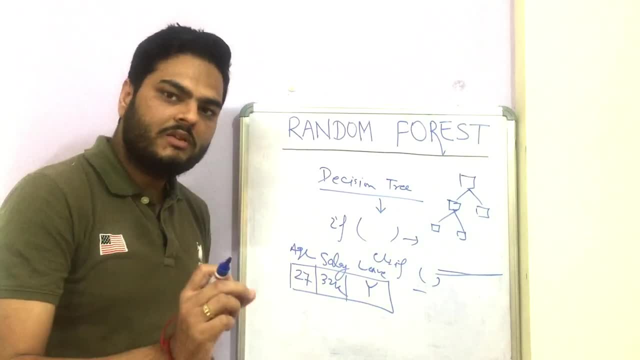 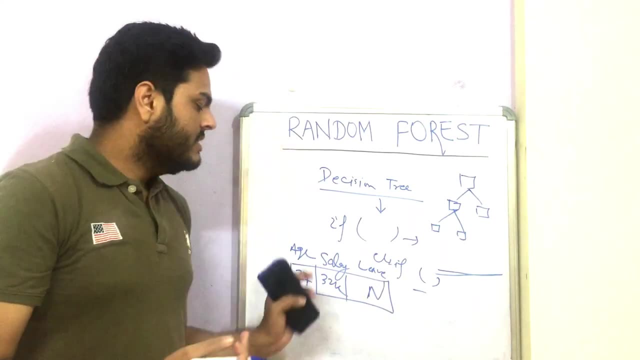 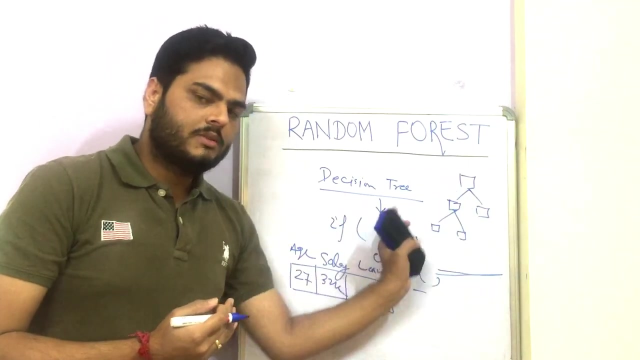 as 27. if you make this 26 as 27, then the test result might change as no, and how it changes is. it is quite possible that if you make that 26 as 27, then it might change the branch in which it goes. So that is how the prediction happens in decision tree. This particular thing is called high. 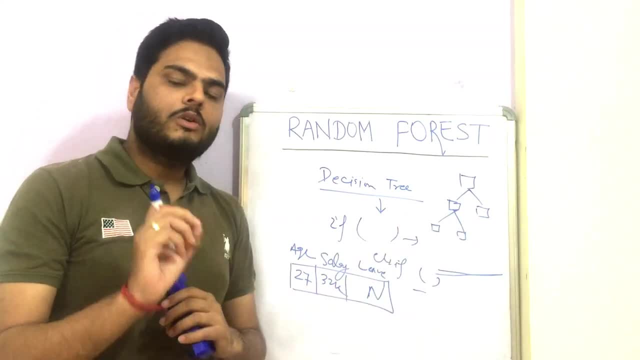 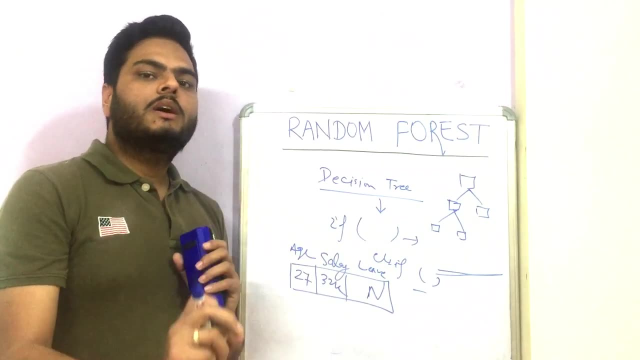 variance of the model when model is doing good on the trained data but not doing that great on test data. So what is the advantage of random forest? Random forest reduces this high variance. Random forest minimizes the variance of the model. How it does that? Let us see how. 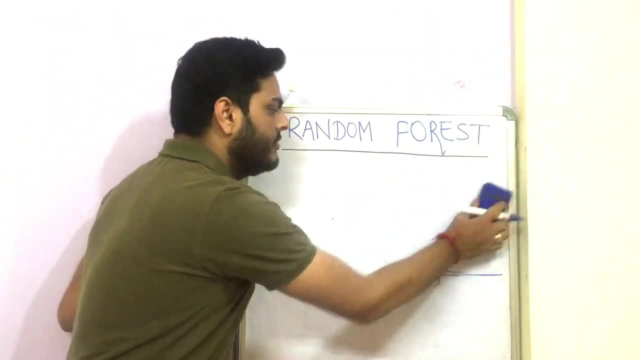 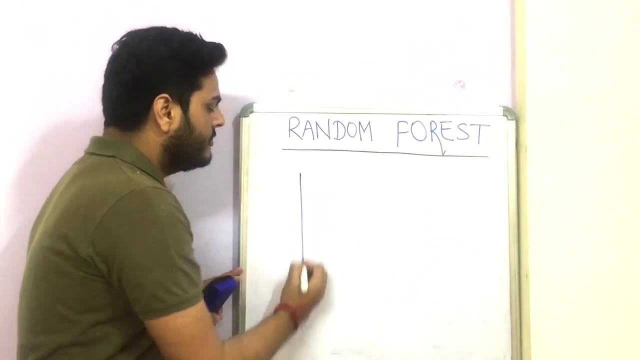 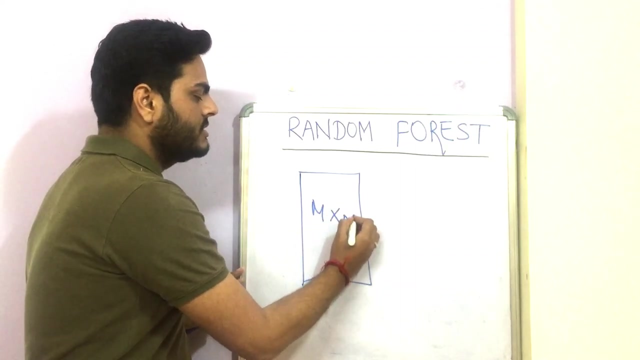 random forest works. okay. So in random forest, the decision trees are built using the bagging technique. okay. So if this is your main data, this is the main data. let's say, this data has m rows and n columns. okay, This is the main data. From this data, using bootstrap aggregation or 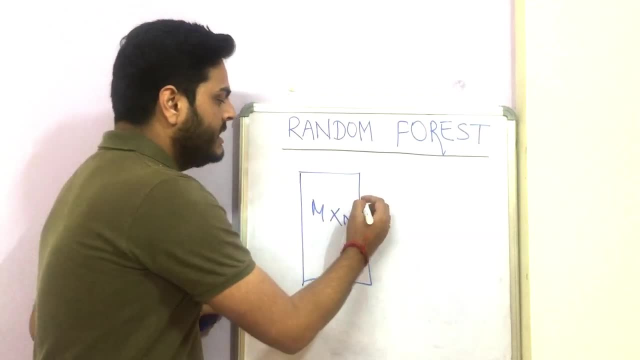 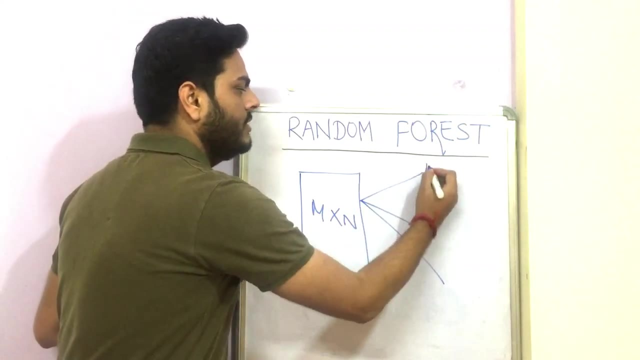 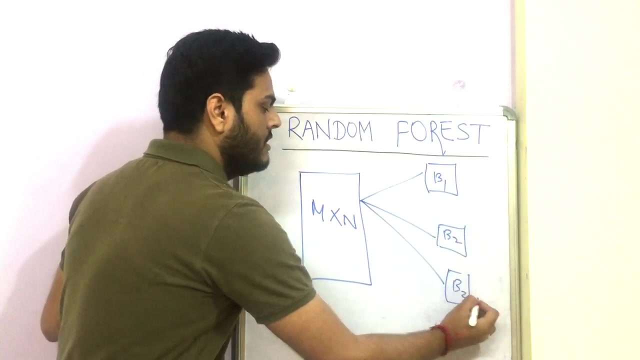 bagging, which I have discussed in my this video. multiple bags of data will be created. For simplicity, if I put three bags here, okay, So this is the bag 1 of the data, This is the bag 2 of the data and this is the bag 3 of the data. For all these bags, there will be row sampling and 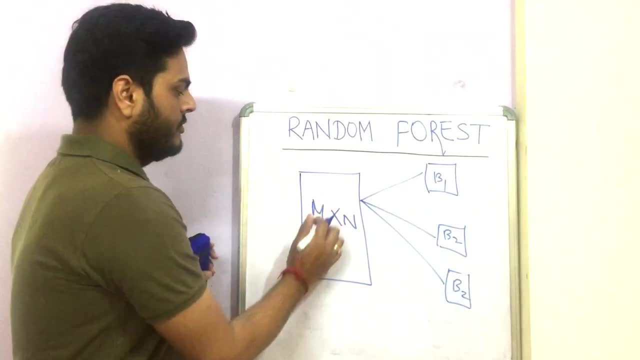 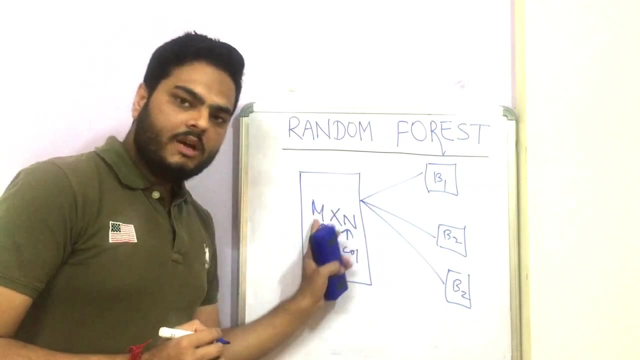 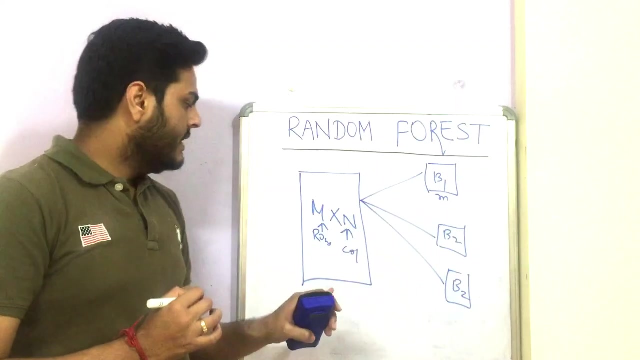 column sampling as well. So what I mean by that is from this m rows, okay. So m is the number of rows and n is the number of columns. From this m rows here m small, m randomly selected rows will come in this bag, okay. And from this n column small, n randomly. 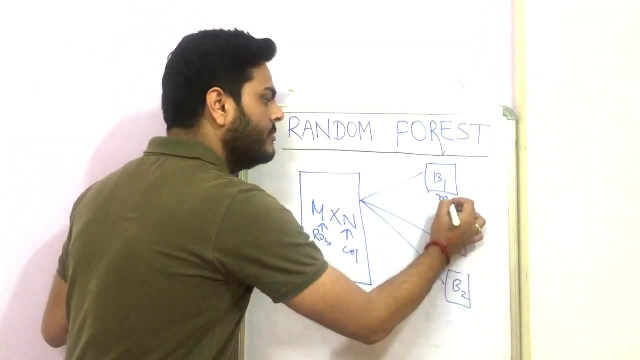 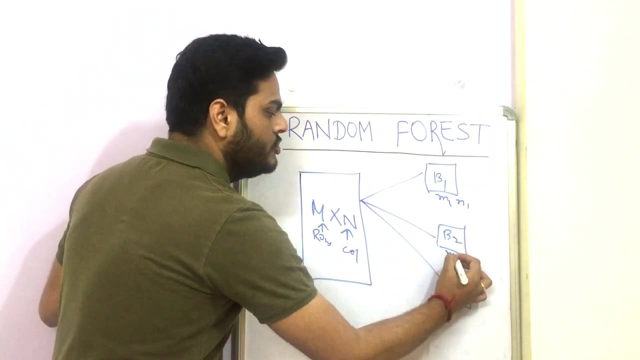 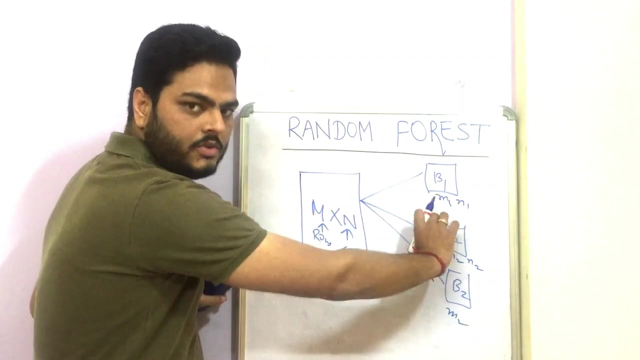 selected columns will come in this bag, So let me make it m1- n1. okay. Similarly, from in this bag, from this data, m2 number of columns and n2 features will come In this bag. m3 columns from the main data and n3- number of rows will come. 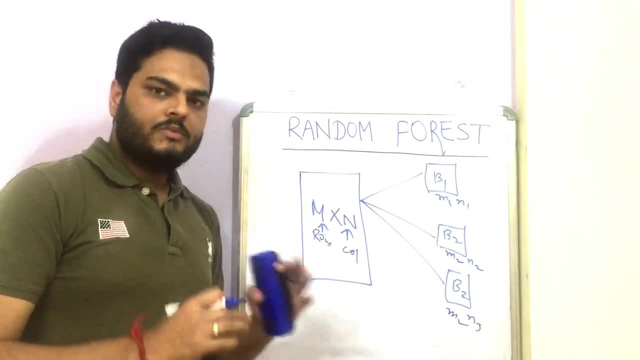 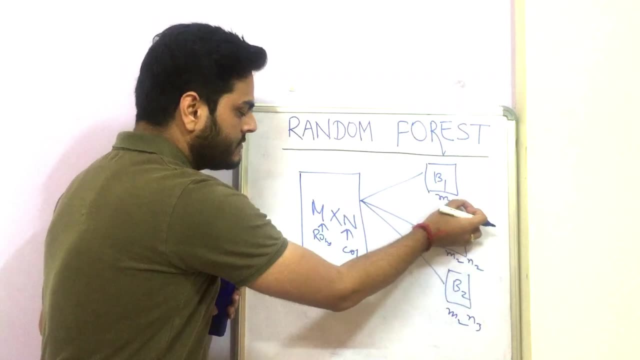 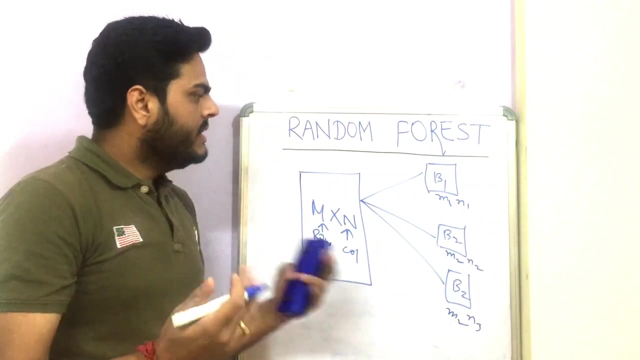 Remember guys always, this small m will be smaller than capital m, Simple right, because it is the sample from the capital n. Similarly, this small n will be smaller than capital n because it's a subset of that. Now, what is the optimal size of this? m1 and n1.. So typically one third of the data. 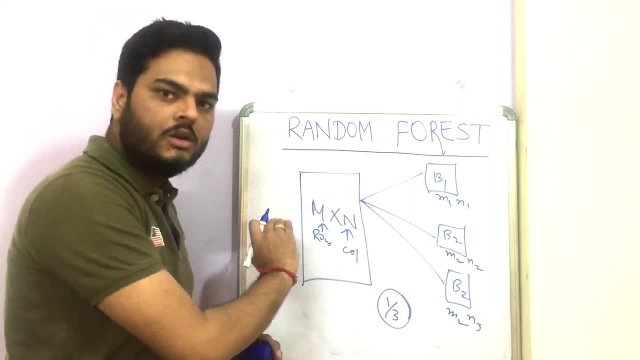 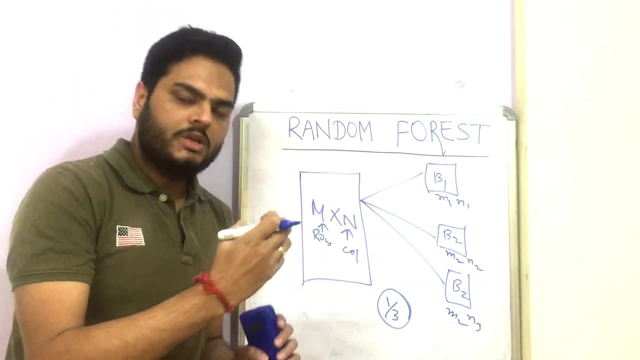 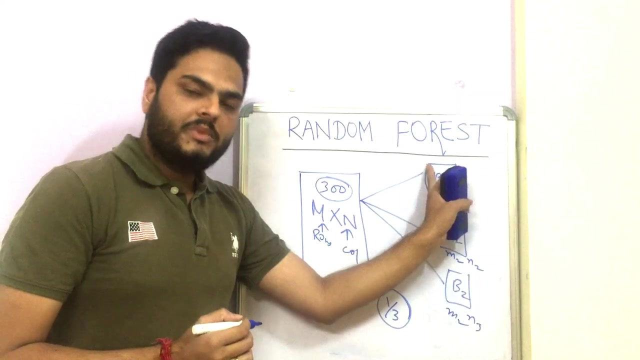 one third of the data in the main data set will not come in this bag, okay, Which means two third of the data comes in this bag, okay? So if we start with 300 rows, then 200 rows will come here. randomly selected 200 rows will come here. 200 rows will come here, And this is a width replacement. 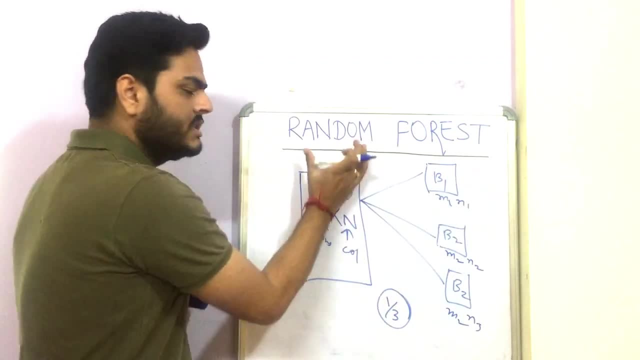 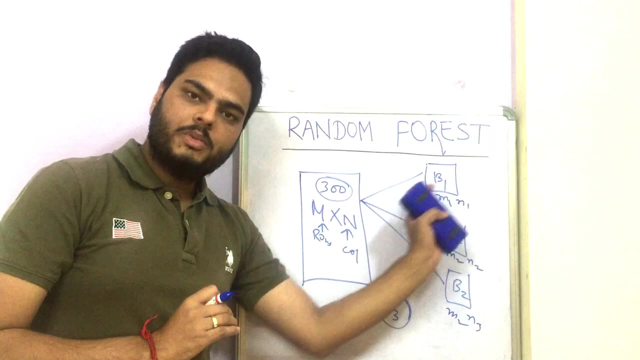 selection, which means, once this bag is created, all the rows comes back here and that is the candidate for coming in this bag as well, Which means there can be repeated rows in this bag and this bag as well. So this is how bags are created, Similarly columns. So how? what is the optimal? 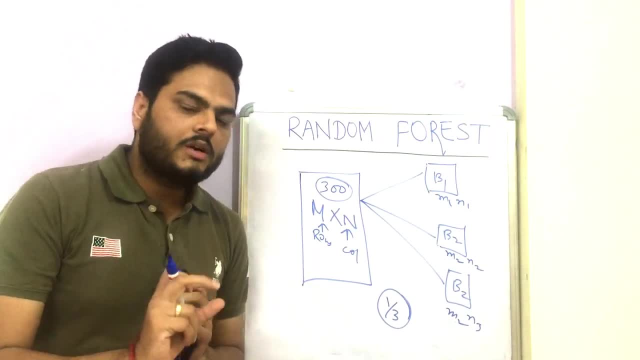 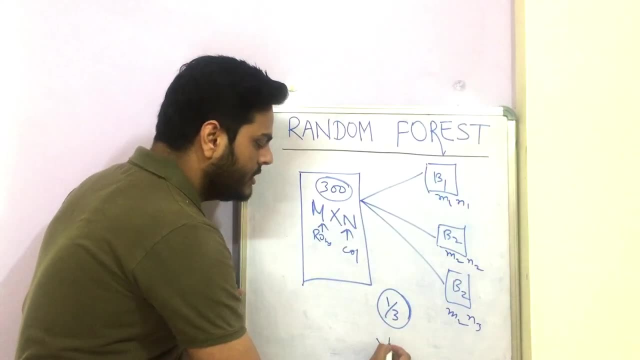 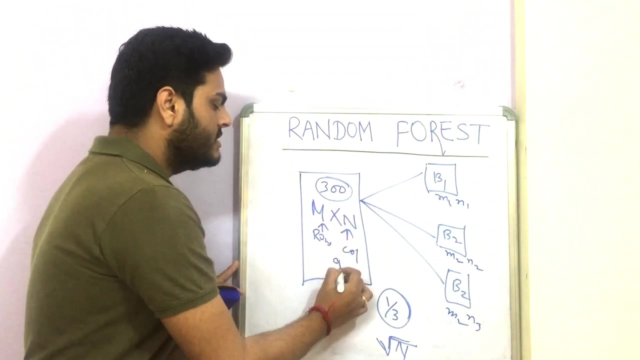 number of columns. So there is no, you know, we can give. this is the optimal number of column we should take. We should, you know, keep changing the number and then decide. But under root, capital n is one, you know, base from where we can start. So if we start with nine columns, then three columns. 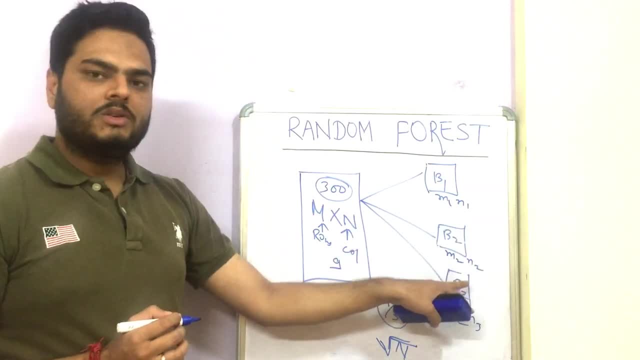 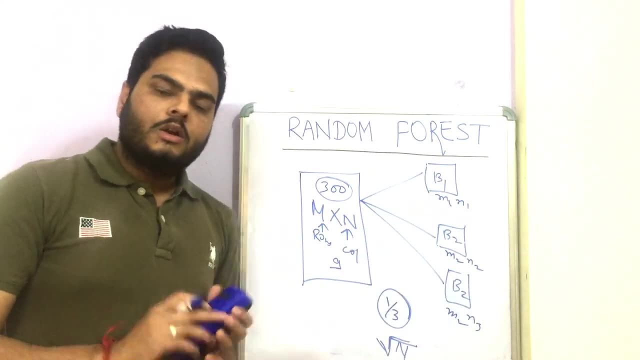 randomly chosen here. Three columns randomly chosen here, Three columns randomly chosen here, Again with replacement, So columns may repeat. So this is how bags are created. Now what happens once the bags are created? One decision tree will be fit on this bag. 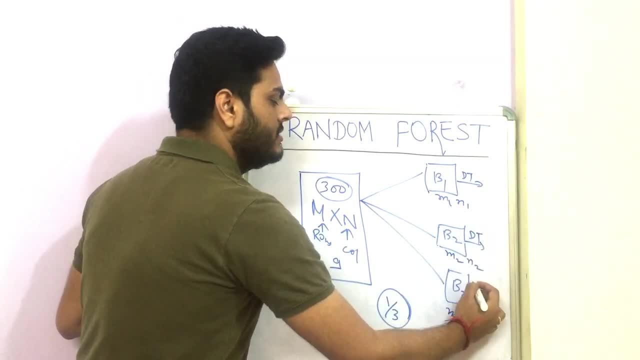 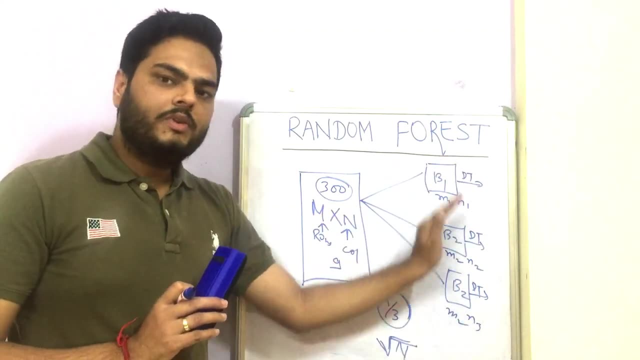 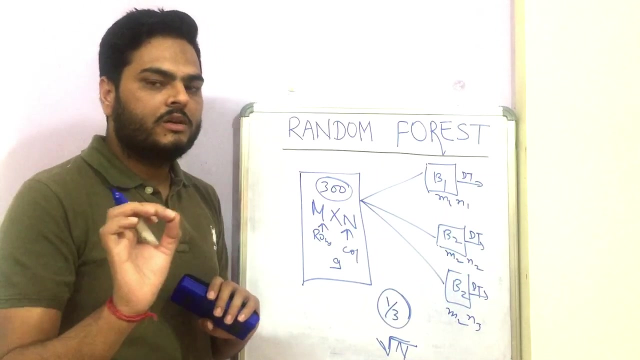 Other decision tree will be fit on this bag. One decision tree will be fit on this bag. Now, when we run a random forest, multiple decision trees are being fit on these bags, Okay. and tomorrow, when a test data comes, when we want to test or predict what is the output. 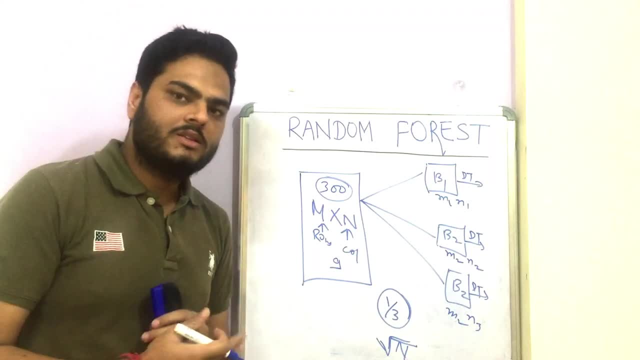 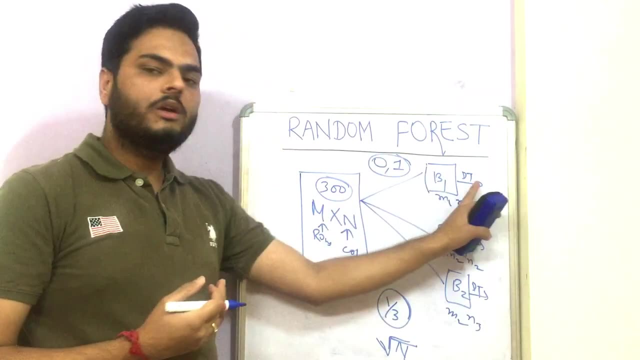 from the random forest. Let's say we are talking about two class classifier. This tree will say: let's say, our target variable can be zero or one. So this tree, when we test on this tree, that happens internally. So I am talking about how random forest gives you prediction. 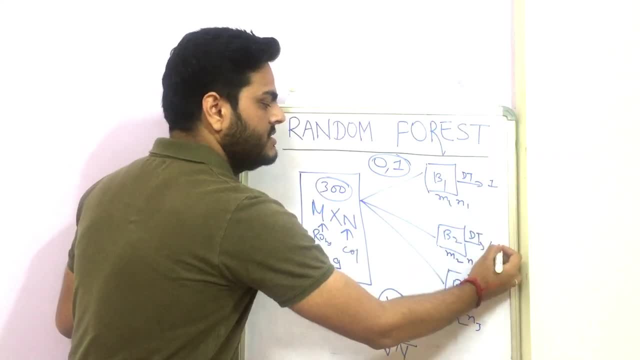 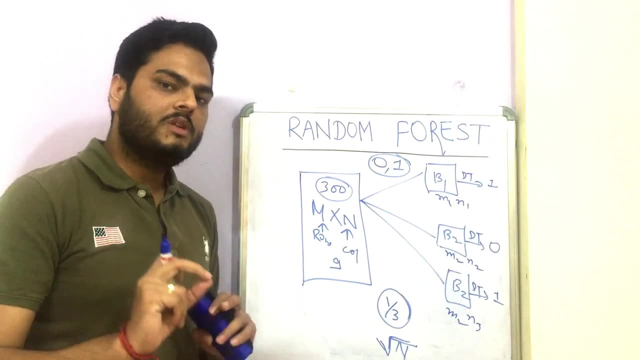 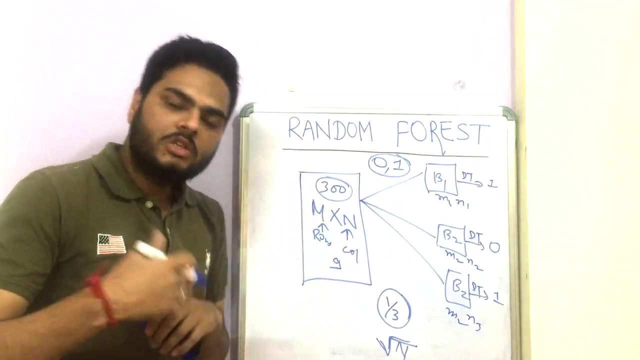 Okay. so let's say this tree says one, This tree says zero and this tree says one. So majority voting. I repeat, here majority voting comes into the picture in random forest prediction. So what is the majority voting here? one. Hence the prediction from the random. 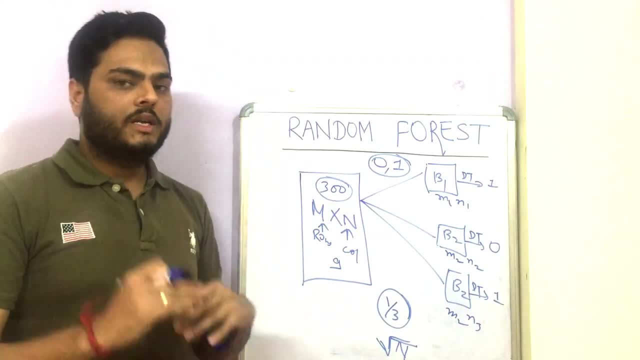 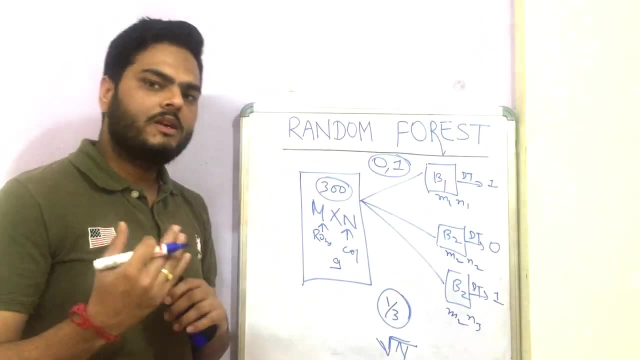 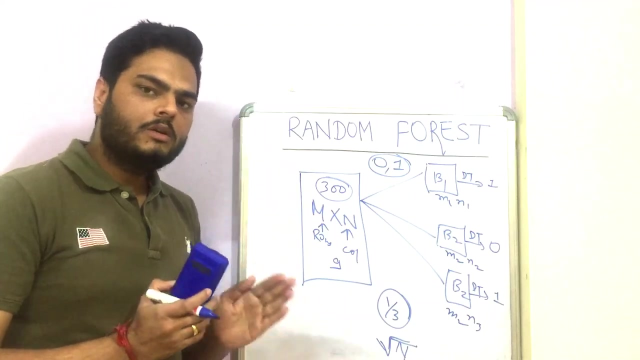 forest will be one. What happens if it's a regression scenario? We can either take mean of all this or median of all this, But in python syscalant, generally mean or average of all the decision tree is the predicted value from the random forest. Okay, so this is how. 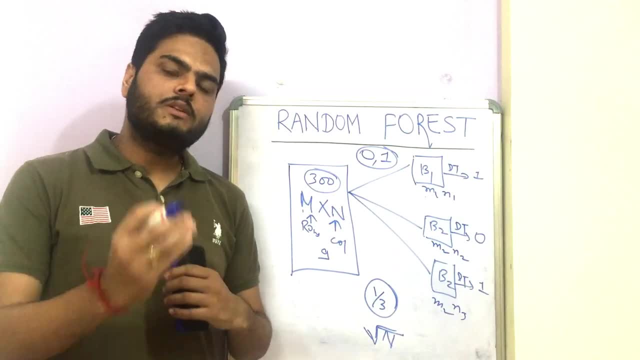 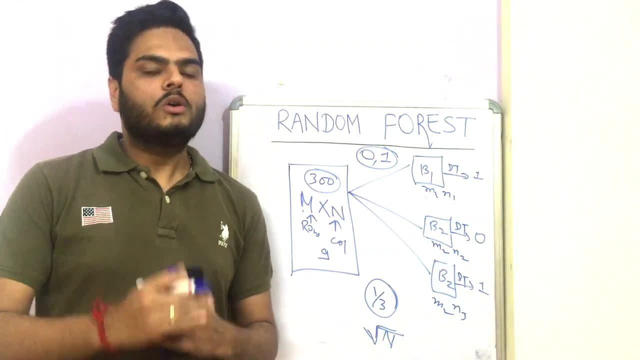 random forest works and this is how the prediction happens in random forest. But why random forest tend to perform so good in comparison to normal decision trees, or why it is favorite for so many people out there. So what happens here? how it reduces the variance. 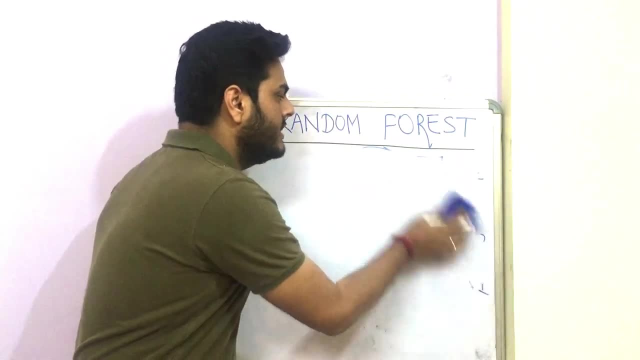 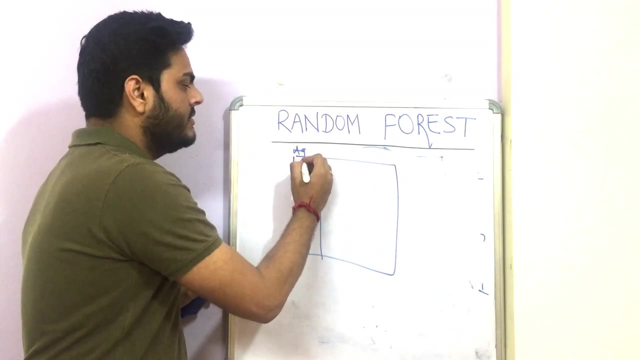 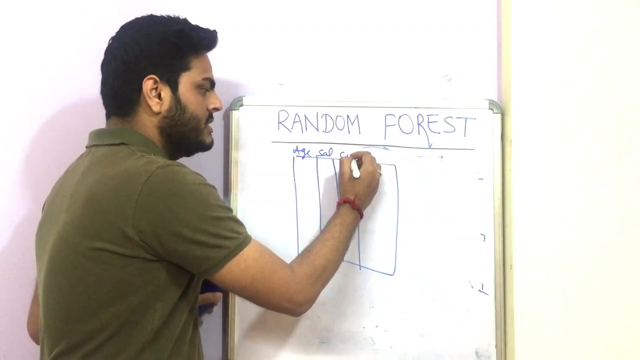 I'll give you an example and try to make you understand. So let us say, this is the data we are working on. Okay, so this is a organization data. Let's say, in organization data we have age- Okay, age of the employee, then salary of the employee, and then you know commute distance. 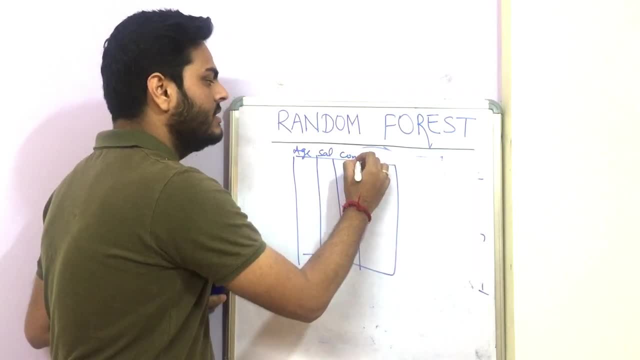 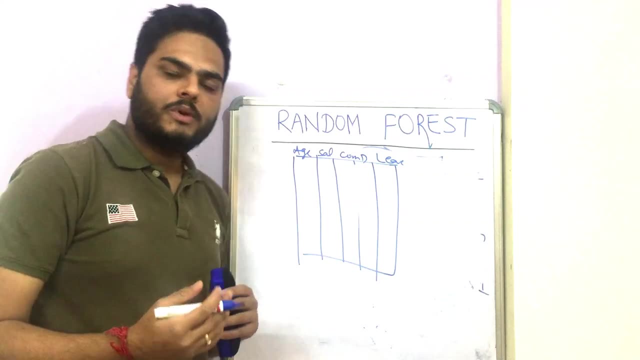 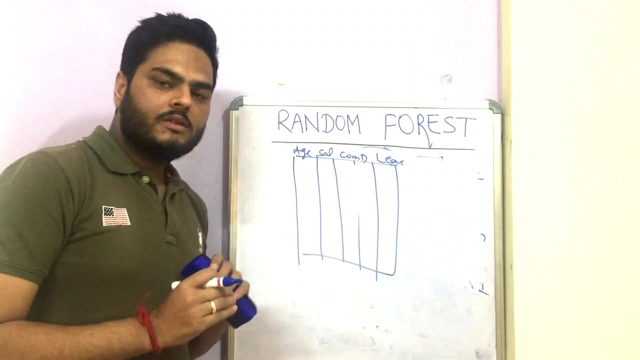 Let's say how much you commute to reach to your office. Okay, so I'll say comm D- commute distance, and then I say whether employee leaves or stay in the company. Okay, so this is the data on which you train your model. Let's say a classification model again. So in this case, what happens? 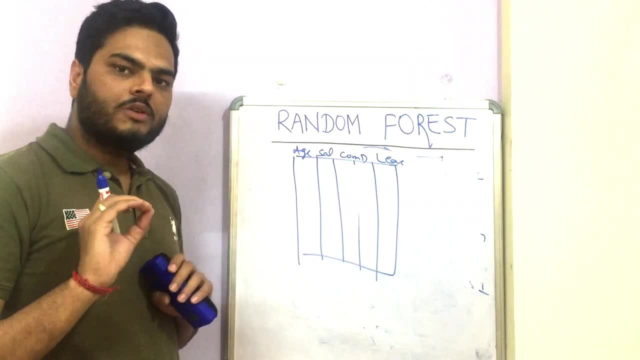 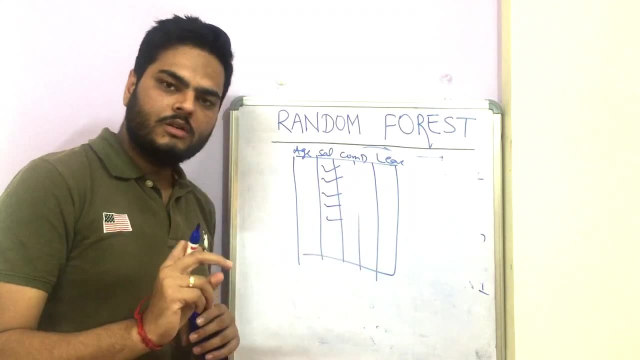 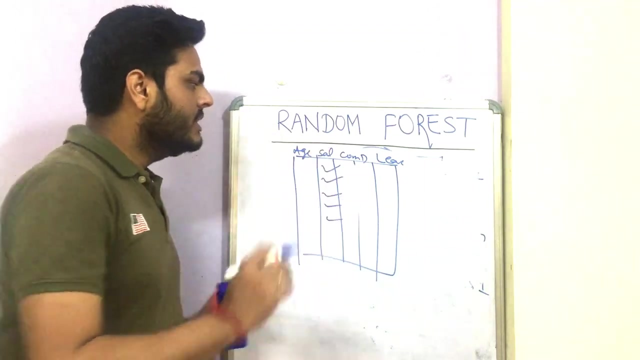 when we take one decision tree only. So what will happen here is: all of us know that salary is a very strong variable for someone to take a decision whether he or she wants to stay in the company or leave the organization- Right. So when we create one decision tree, 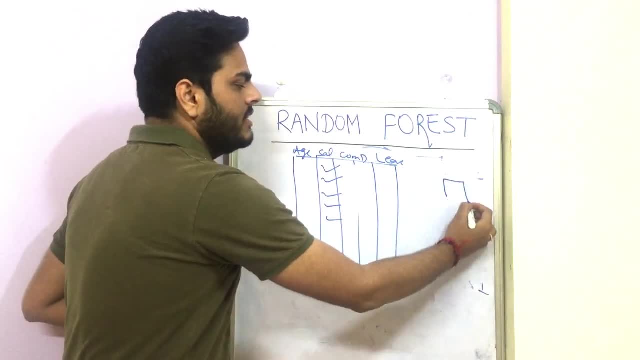 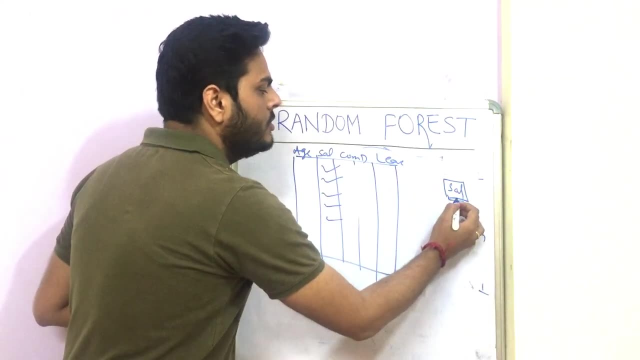 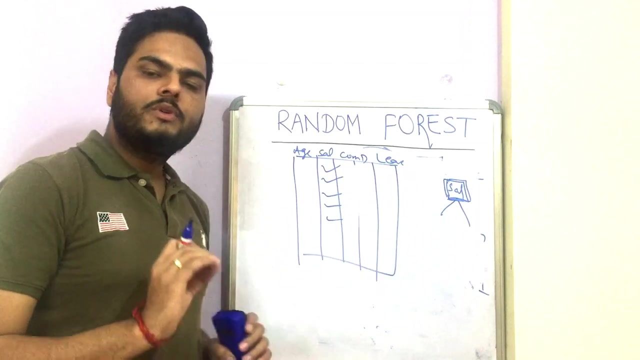 salary will always come out to be a strongest variable or, in terms of decision tree, it will be root node mostly, which means strongest variable. So what happens when we test on, you know, when we predict or test on the trend model, is every time the salary, the salary. 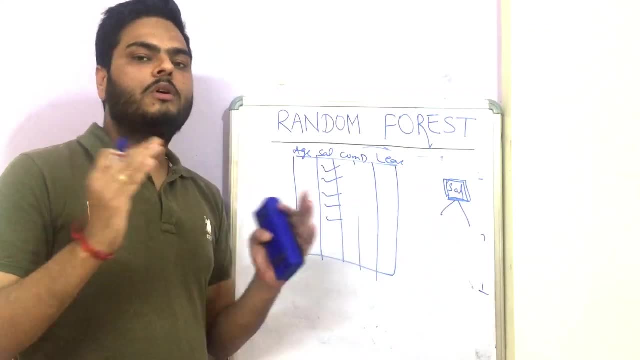 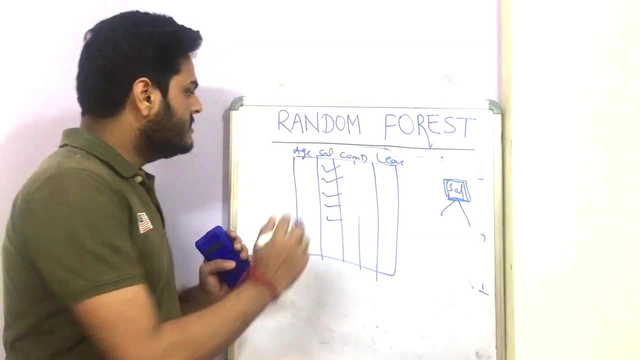 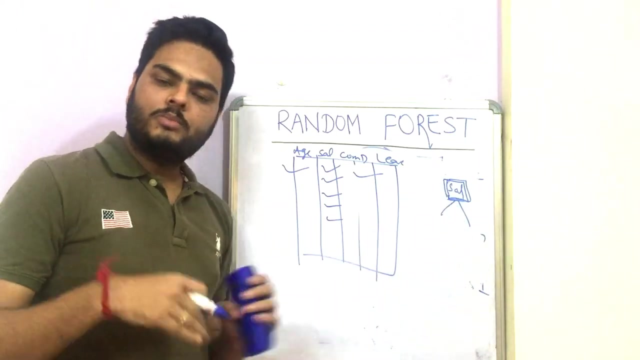 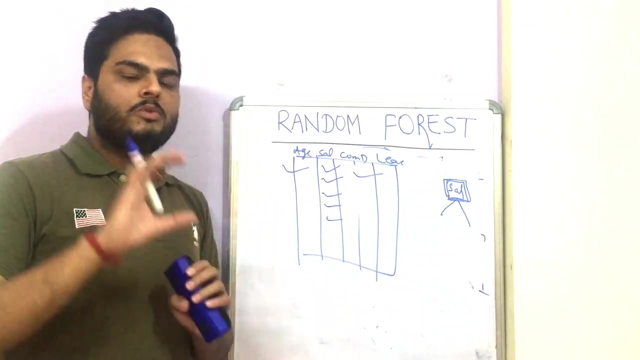 feature dominates the behavior of all other features. So just try to understand. Okay, Salary is a very strong variable and hence all these variables is your commute distance. These variables also may be important, but salary is so important that every time you test or try to predict on this trend tree, only salary is going to contribute to the 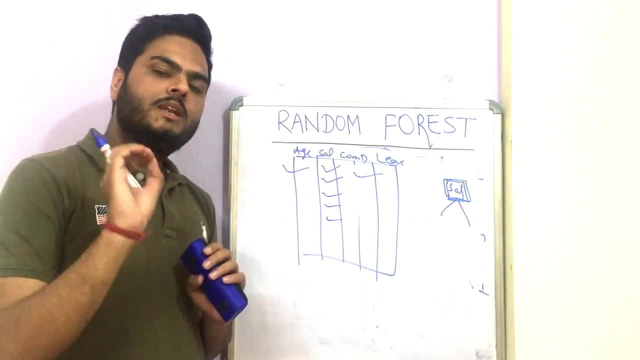 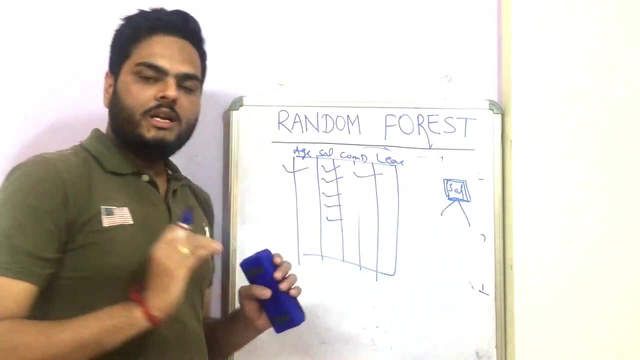 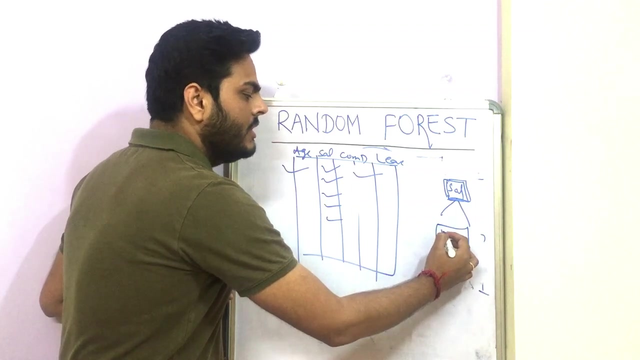 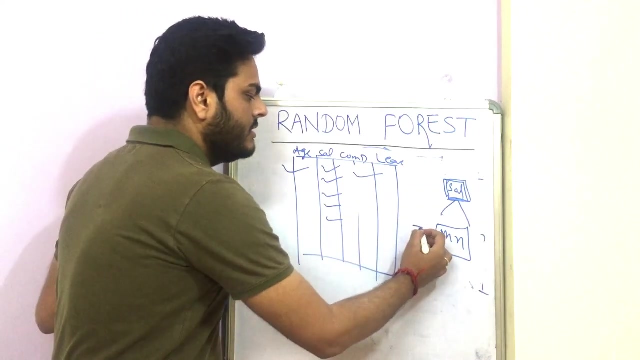 decision to a very high extent, and hence salary suppresses the effect of these variables. But what happens in decision tree is when you create multiple, Multiple trees, Right. So this tree may have, as I told, in my picture, all the trees will take M rows and N columns, which are subset of the main data. Now, this is tree one or 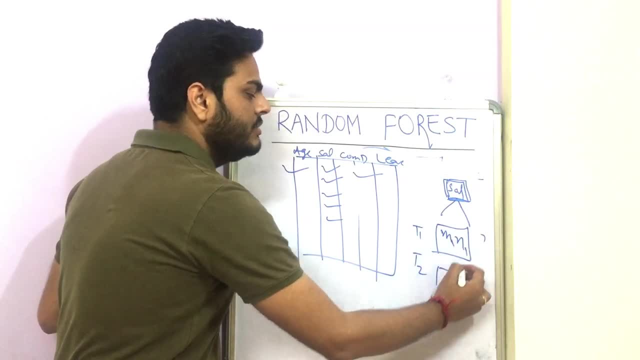 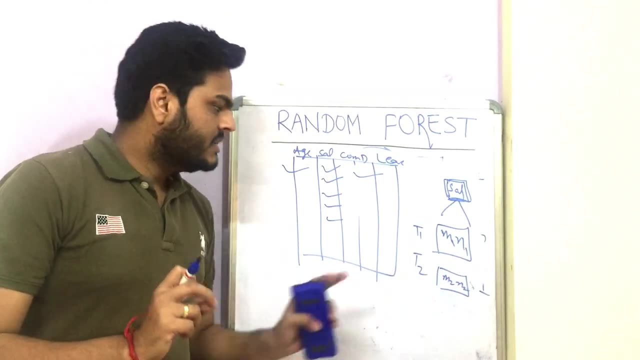 bag one. the tree two is built using this is built using M1 and one. this is built using M2 and two. There is a high possibility that in one of these trees salary is not part of the feature And hence the training happens on other features. 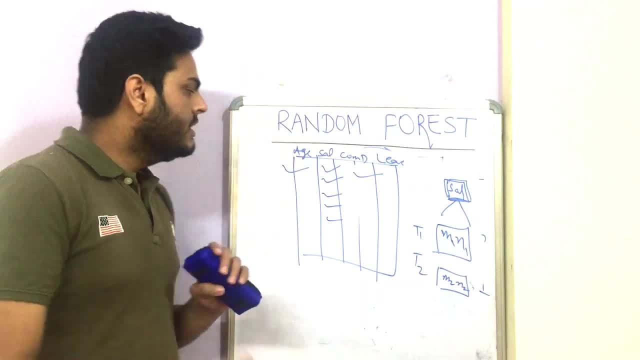 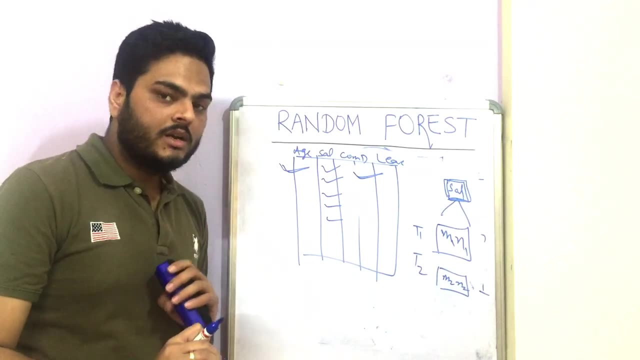 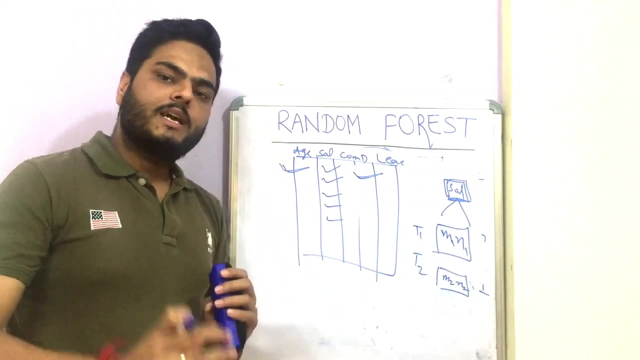 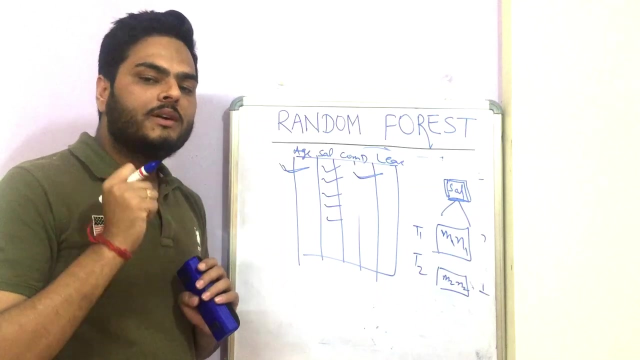 So other variables. what will happen in that case is any learning, any pattern in age column or commute distance column will also be captured and that particular tree also votes in the final decision. and hence random forest captures the pattern of the data from various angles. That is why random forest always tend to give you good result. What are the other advantages?